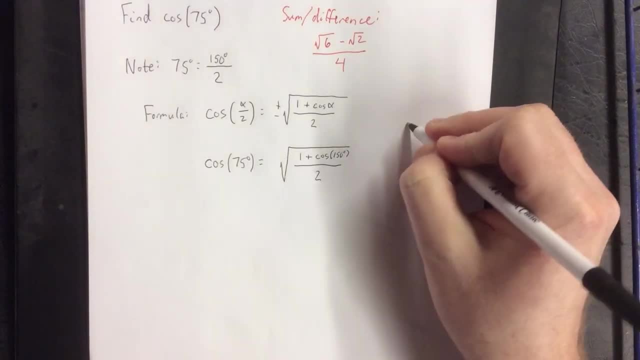 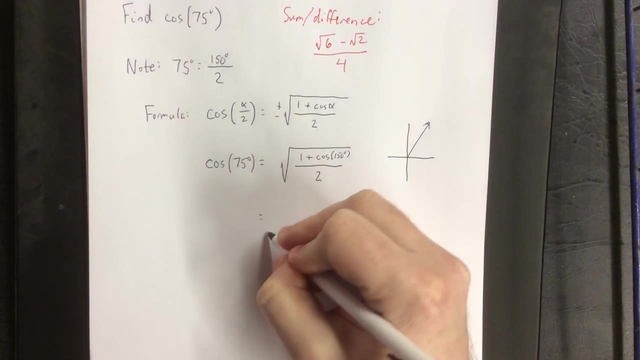 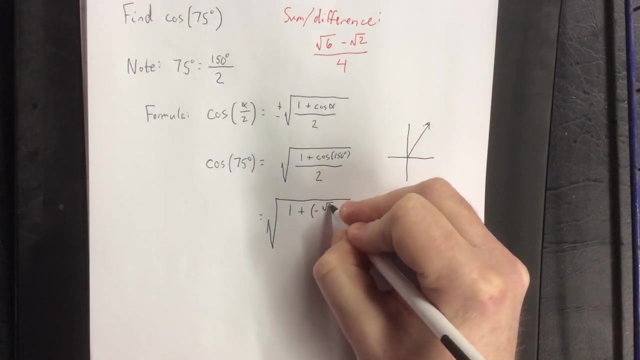 minus anymore. This is because I know 75 degrees as quadrant 1 angle and in quadrant 1 the cosine will be positive. Now to simplify this further, this will be 1 plus cosine of 150 degrees comes from the unit circle that'll be negative square root of 3 over 2.. This is all. 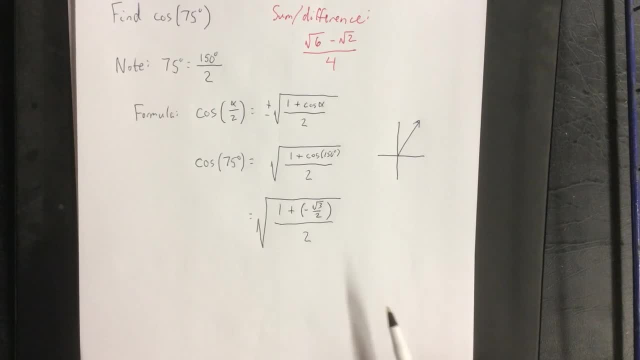 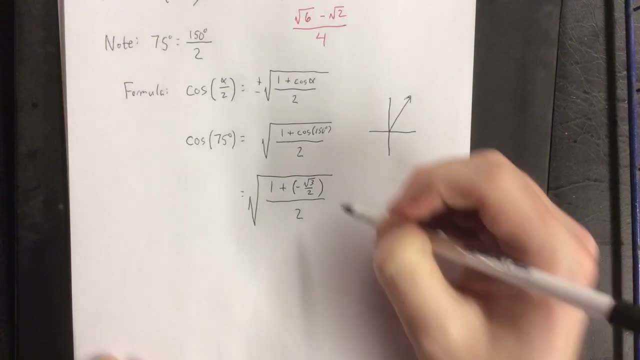 still over 2.. Yo dawg, I heard you like fractions and radicals, so I put a radical inside of your fraction, inside of your fraction, inside of your radical Boy. that just sounds like a good time, doesn't it? Well, here's what I'm going to. 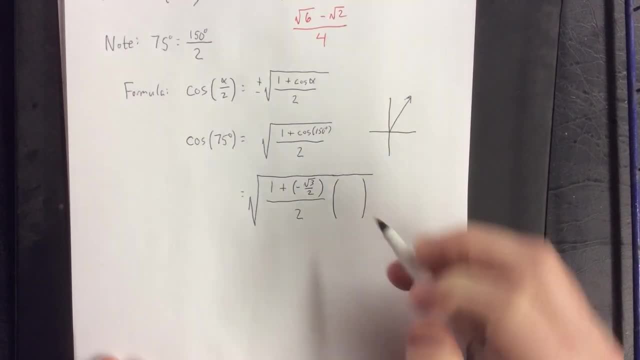 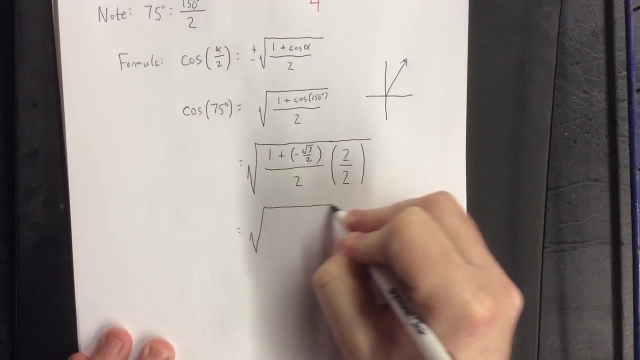 do in response? I want to at least clear out the fraction. I want to at least clear out the fraction inside the fraction. So I'm going to multiply the big fraction by 2 over 2.. Upon doing so, that will distribute through the. 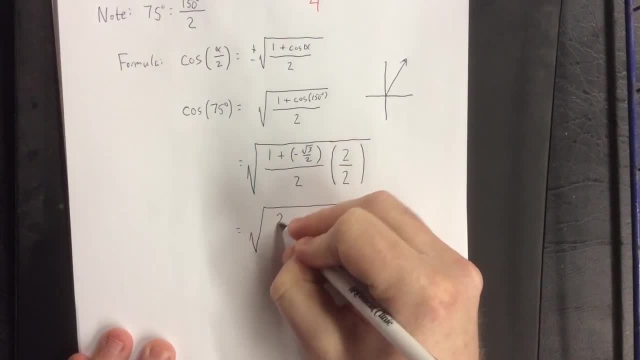 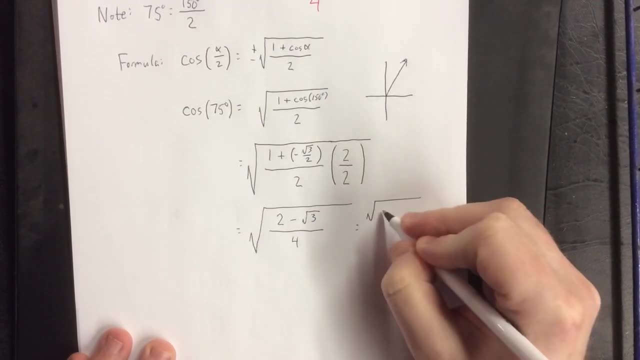 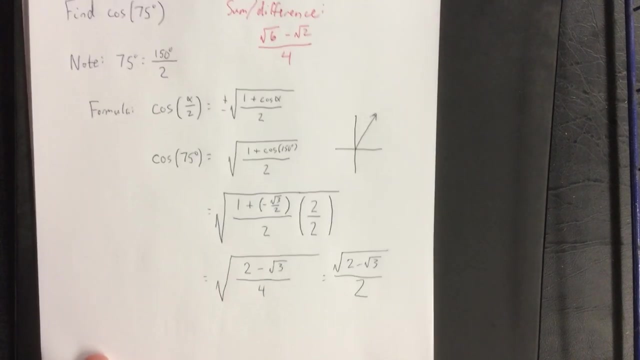 numerator. We'll call that 2 minus the square root of 3 in the numerator and then the denominator 2 times 2 is 4.. The only further simplification that I want to do is in the denominator by taking the square root of 4.. Now compare this. 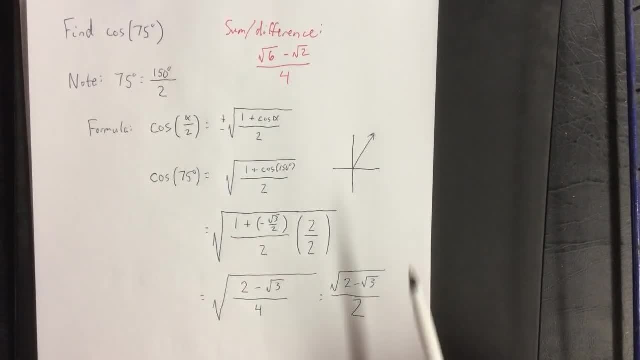 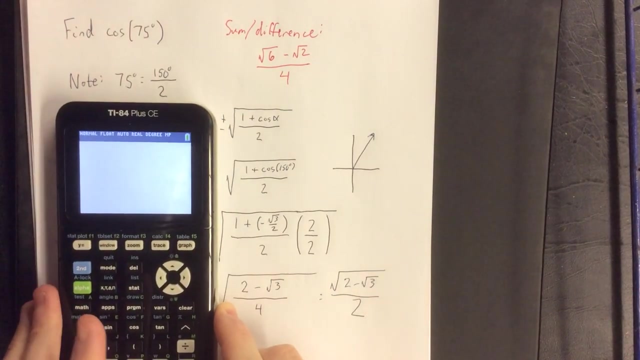 answer the square root of 2 minus root 3 all over 2 with the answer that we got the other method. These two numbers look basically nothing alike, So that's kind of disturbing to me. But what the heck, Let's go for it anyway. Let's take the square root of 2 minus the square root of 3 and 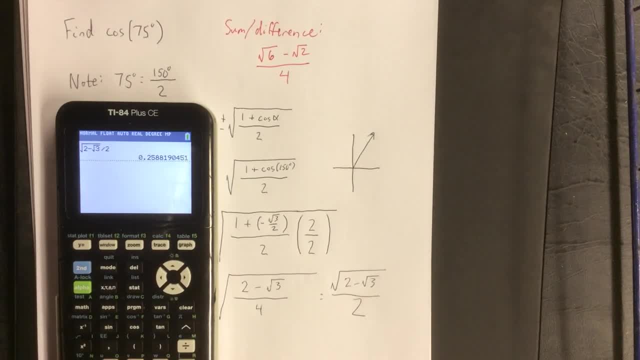 put that whole thing over 2.. Ok, and then let's try plugging this into the calculator. So big set of parentheses for the whole numerator, all over 4,. what do you know? They happen to be the same number, and in both cases that is equal to the cosine of 75 degrees. So if you 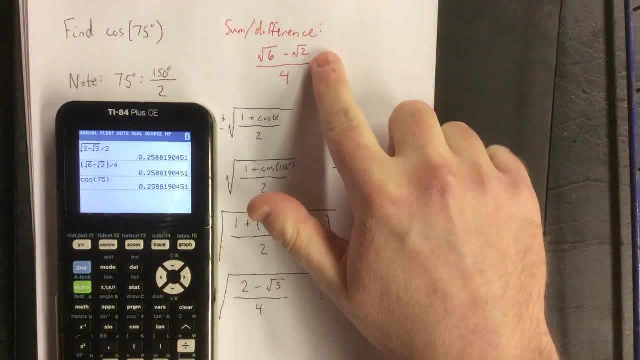 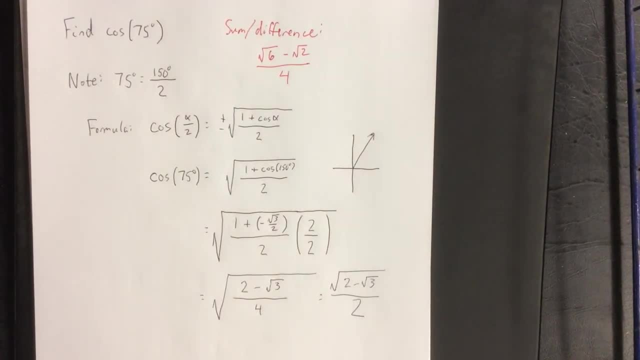 and a friend are both trying to find the cosine of 75 degrees. one of you tries a sum and difference identity and one of you tries a half angle identity. it doesn't mean that either one of you is wrong. It just means that you took on a.